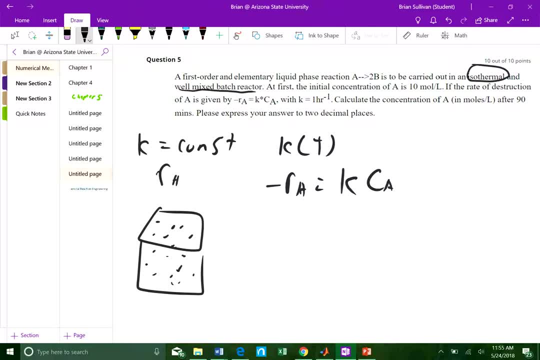 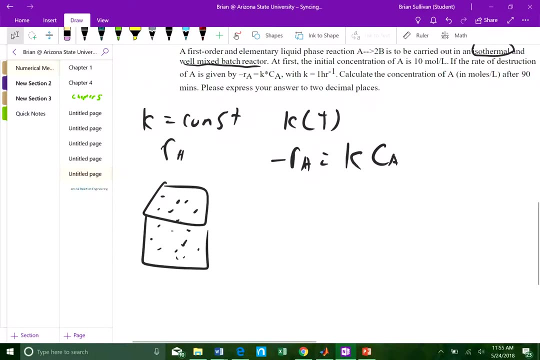 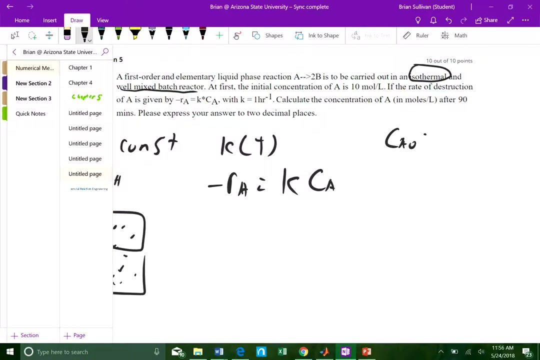 And in this case it's going to be first order. So the concentration is the same everywhere else, everywhere in the reactor. So this will be the same everywhere in the reactor. That's the way to think about that. Now you're dealing with first order, elementary liquid phase reaction, So it's going to be KCA. Okay. so let me drop down over to the right over here and write down all the variables that were given. So the initial concentration of A is 10 moles per liter. So they give you this structure. 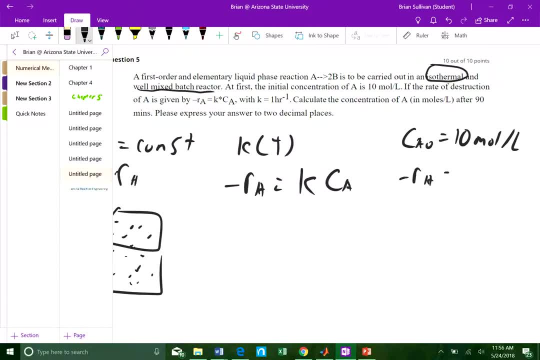 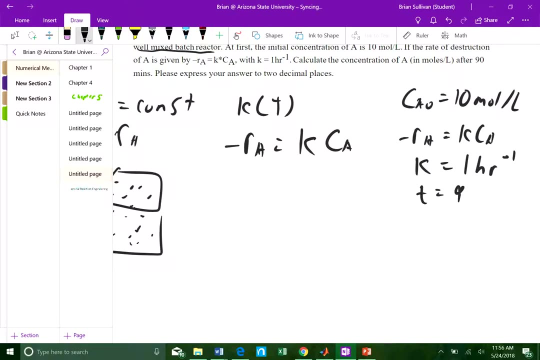 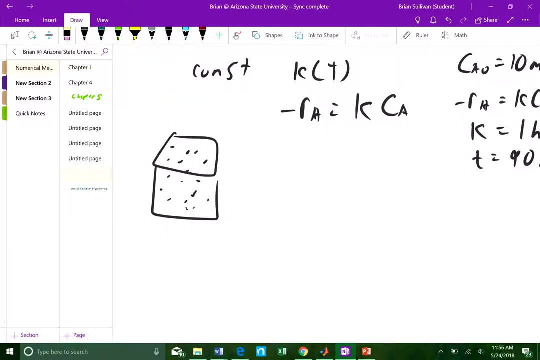 So the initial concentration of A, which is right. here we have it, I'll write it anyway. RKCA, And they give us the rate constant. Calculate the concentration of A after 90 minutes. Okay, so T is equal to 90 minutes. That's how long our reaction is going to go for, Okay. so let's keep these in mind. I'm going to clear up some room. I might leave the box there, just to keep in mind it's a batch reactor And we'll do our analysis. 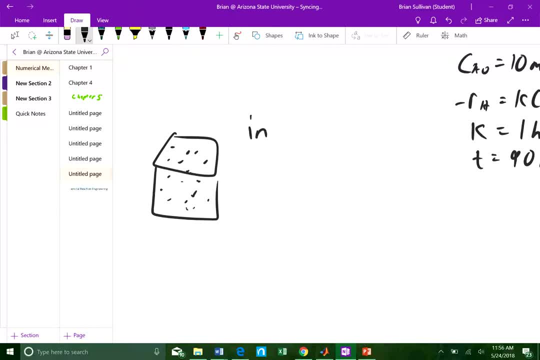 So the first thing you do is you do a mass, a material balance In minus out. plus gen equals accumulation. Now, in terms of a batch reactor, like I said in other videos, you know nothing goes in, nothing comes out during the time of 90 minutes. So you're in and you're out because you've got a lid on your batch reactor. This leaves you with a generation term equal to accumulation. 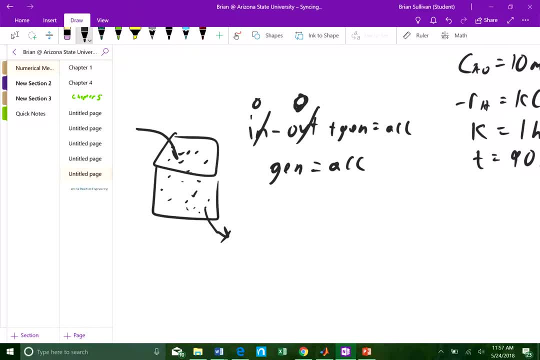 Now, what do we put in for our generation? Now, it was a long time ago, I did this in a video, But that's going to be the, The rate of reaction times, V, And then the accumulation term is going to be the derivative of the number of moles of A over the number of moles. 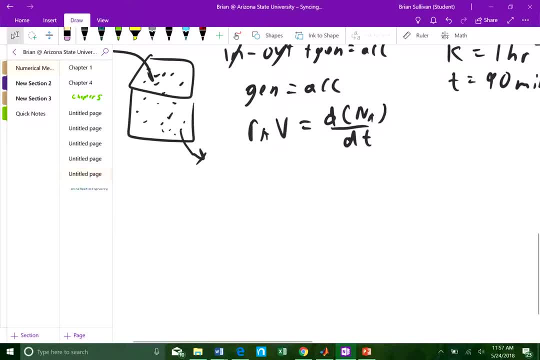 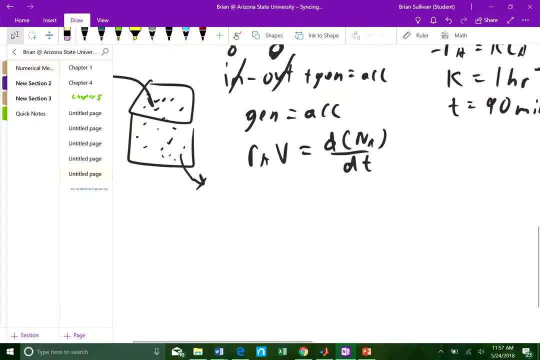 Or not the moles, but the differential time Right. And you can refer back to that first couple videos I did on batch reactors where I discussed why this formula makes sense. Okay, So we're solving for time. So are we giving initial amount of moles? 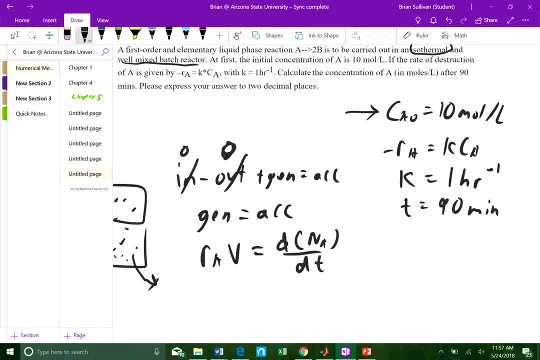 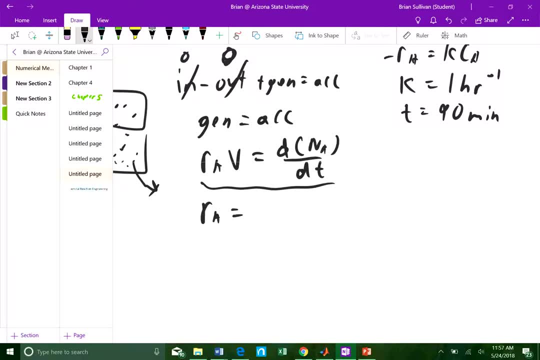 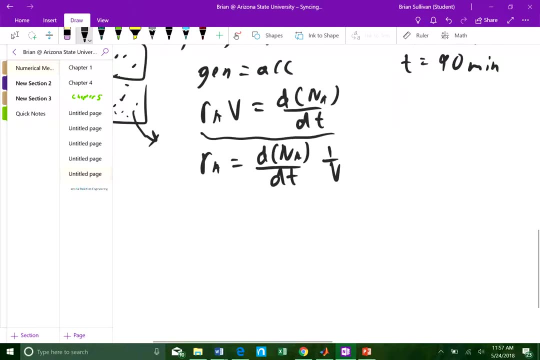 No, we're not. We're not even giving the volume, so we couldn't get the initial amount of moles. But we can make this whole formula in terms of concentration by dividing volume to the other side. Right, Okay, So we move down this way. 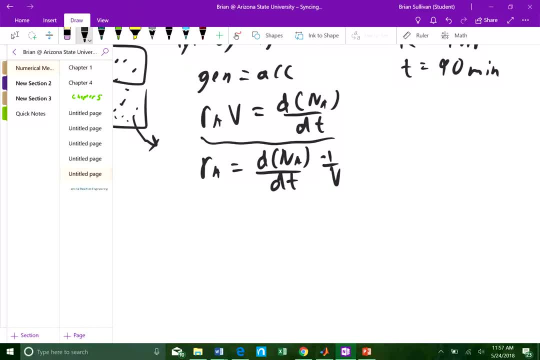 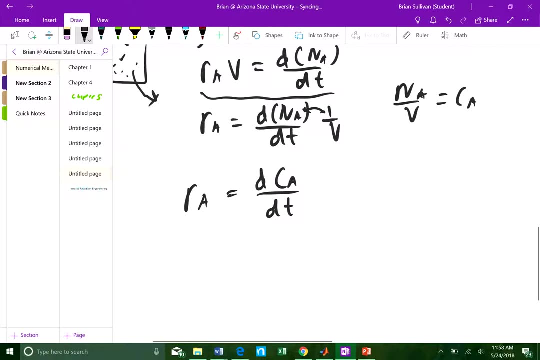 Since V is constant, the volume is constant for a rigid batch reactor. we can put that into the differential term Right: By dividing N A over V, you're going to get C- A. Okay, moving forward, Now we got this equation. 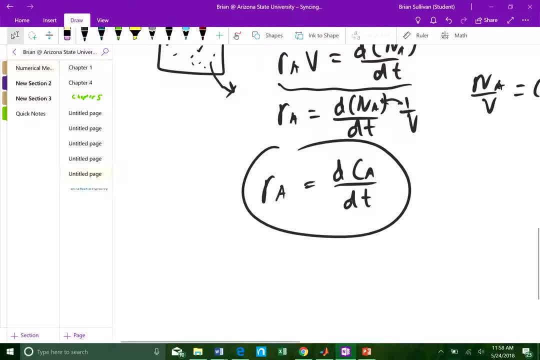 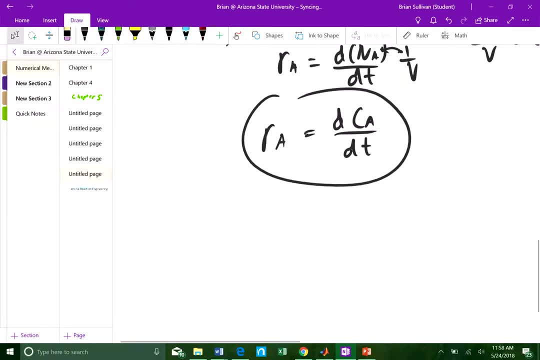 Now, that's something we can solve Right, So let's plug in our first order reaction into R A. Remember, this is positive R A that we have here, So what we're going to want to do is put in negative K, C, A. 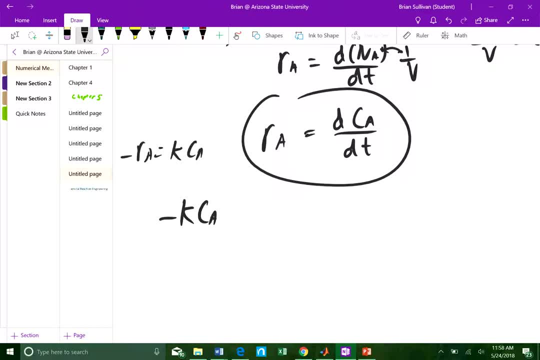 Because negative R A is equal to K C A And therefore R A is equal to negative K C A. And here we have a positive R A value. So negative K C A is equal to D C A Over D T. So push D T to the left side and push C A to the right side. 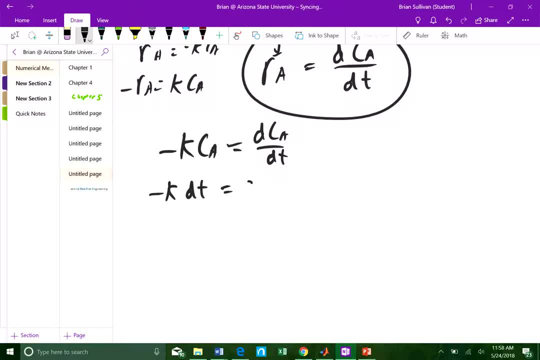 So, then, what you end up getting is this: Alright, So we're almost there. So let's integrate Negative K from 0 to T, D, T. It's going to be integral from your initial concentration that you added, which will be higher than C A. 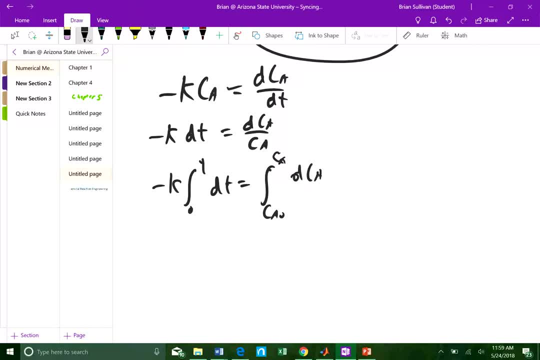 Right, Because you're losing A And this is going to be negative A, So it's going to be D C A, C A. Now if we do the integral- I'm going to right arrow, to the side- You're going to get negative K T. 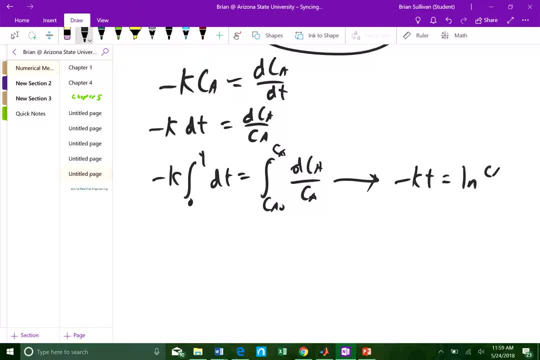 It's going to be equal to the L? N of C A over C A sub 0.. Now to get rid of the natural log, you've got to put both sides as the power of E, So in this case E negative K T. 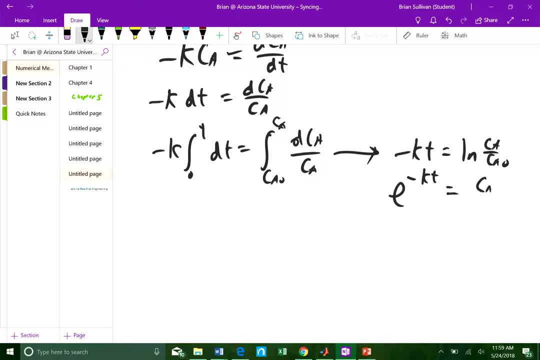 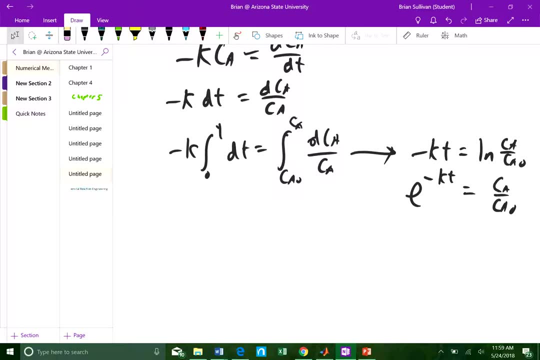 And E to the natural log of C A over C A O. It's just going to give you C A over C A O. Now what we want is: We want this whole formula in terms of C A, So we can plug in the time we were given. 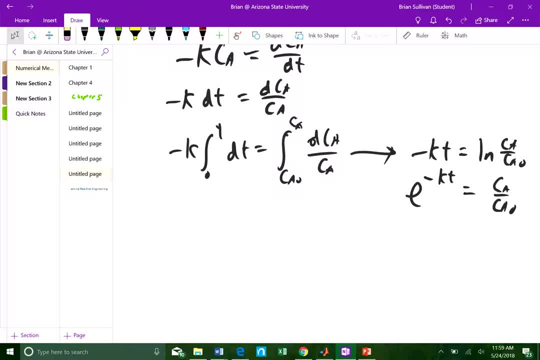 And simply get a concentration after 90 minutes. Okay, So multiply C A, O to the left hand side, E to negative, K, T, It's equal to C? A. So let's bring down our variables, that we know. We know our K. 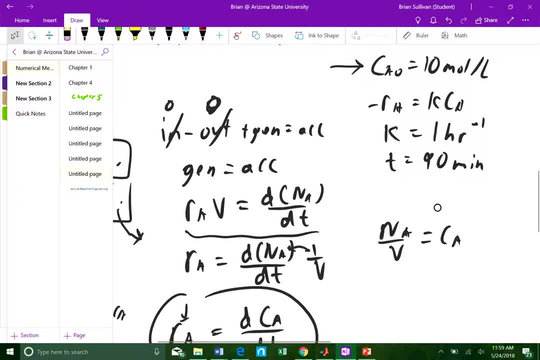 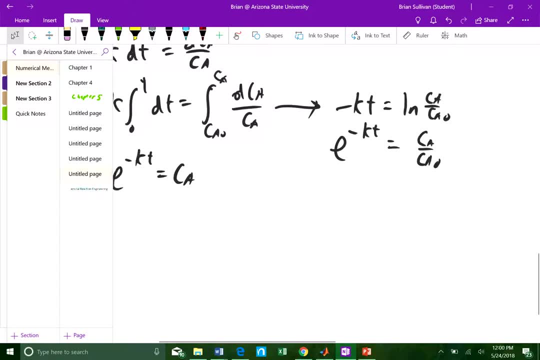 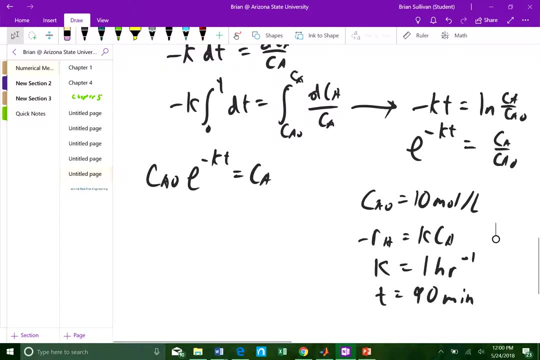 We know our C, A, O And we know our T, So good thing, I'm using OneNote. Okay, Copy this. Bring it down here Easier when you're doing paper on the test, Believe me. Okay, Now These are our variables. 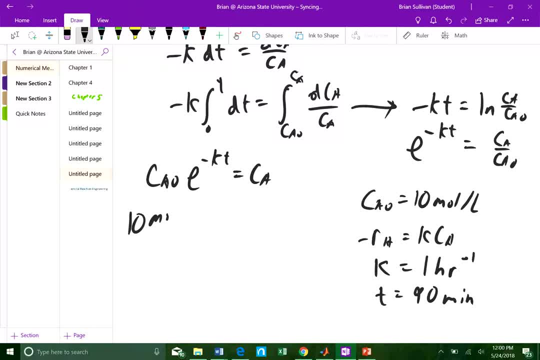 So let's do 10 moles per liter And remember to keep the units alive, Because you're going to see it might make a big difference, And it does. in this case It does Negative 1 over hour Right here. 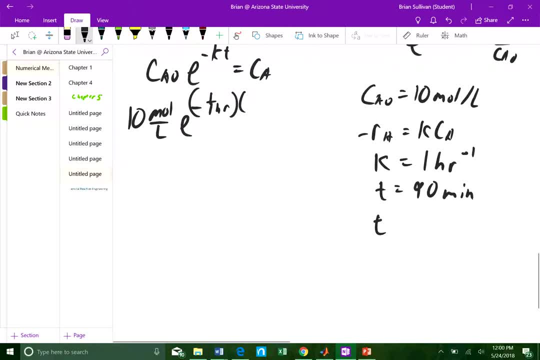 And this is going to be 90 minutes. So let's convert minutes to hours, So that's going to be 1.5 hours, Right? So this will be 1.5 hour. Now the units make sense And it will actually give us a concentration in terms of moles per liter. 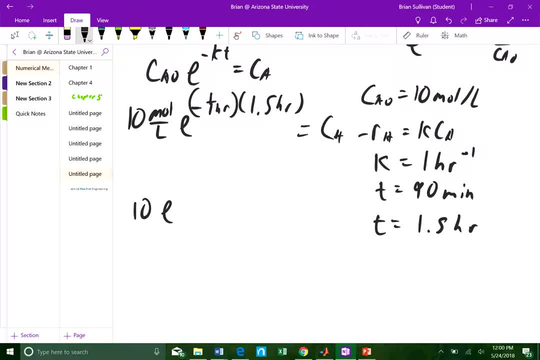 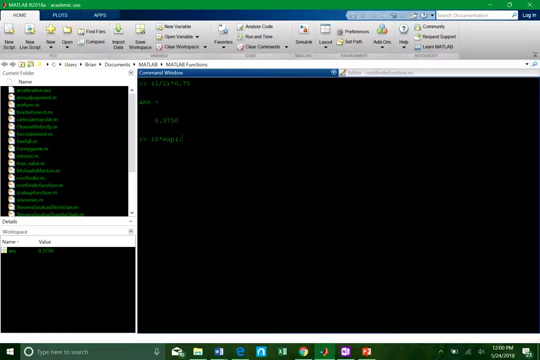 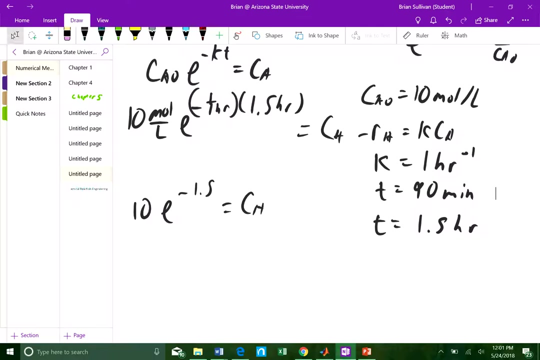 So then let's do this. What is it? Negative hour, So negative 1.5. here You go. C A. Now I'm going to do this in MATLAB real quick. That should be negative. There you go, 2.2313.. 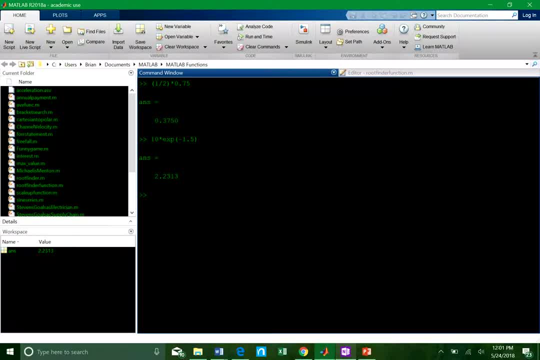 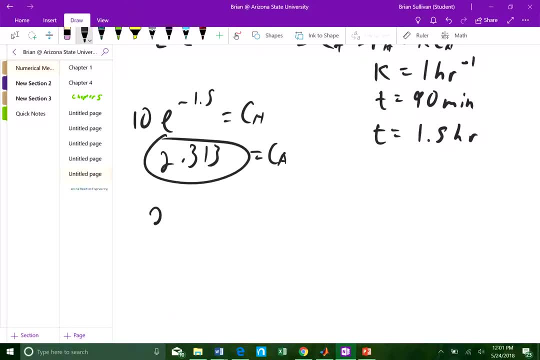 Okay, I hope this helped guys Make sure I did it right. Yep, Everything is good. So this would be your concentration. And what units do you have there? We have moles per liter, Per liter over C A. Now it's important to analyze. does the answer make sense? 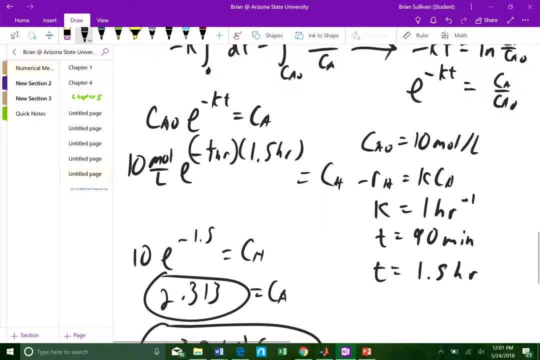 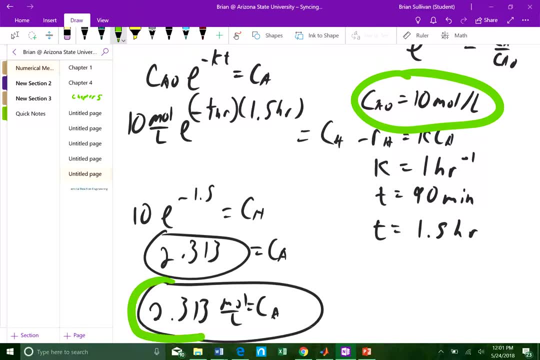 Well, I know that the final concentration should be less than the initial concentration, And indeed it is. It actually cut down- Let me use colors. It cut down by one fifth approximately. So 2.313 moles per liter is equal to C A. 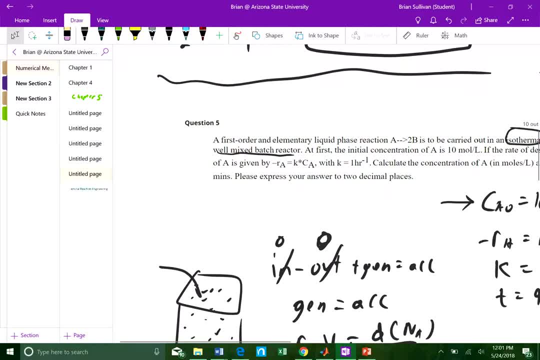 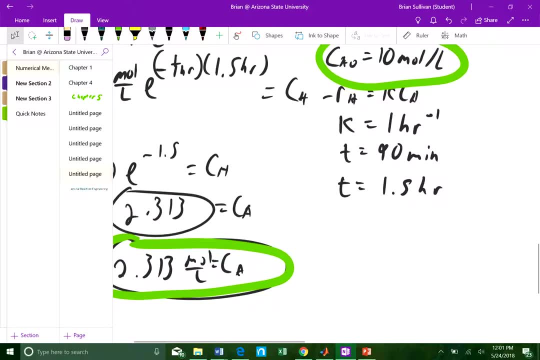 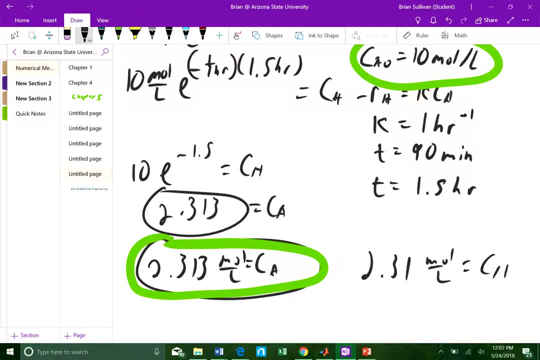 It does make sense And I always check in this class and the answers make sure it's the right decimal places. So it should have been two decimal places. So 2.31 is really what you should have gotten. Okay, I hope this helped, guys. 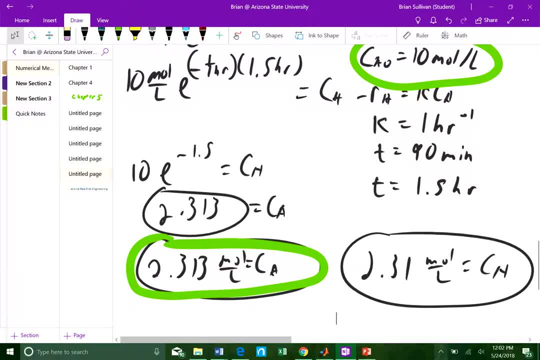 See you in the next video. I'll do even harder ones. Push on guys, Alright. See you, guys, in the next video.